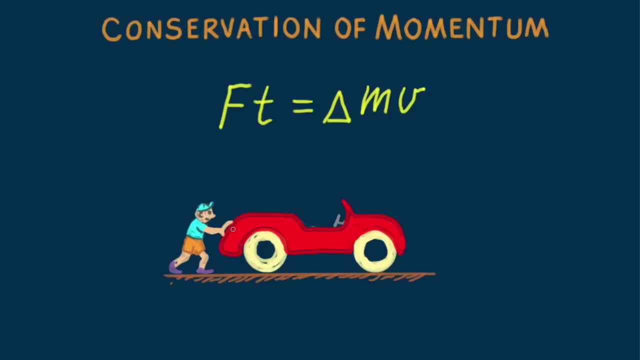 in momentum occurs: None. No change in momentum means that a stationary auto remains stationary and a moving auto continues in whatever motion it has. The same is true for cars, grocery carts or whatever. No impulse, no change in momentum. This relates to inertia in Newton's first law. 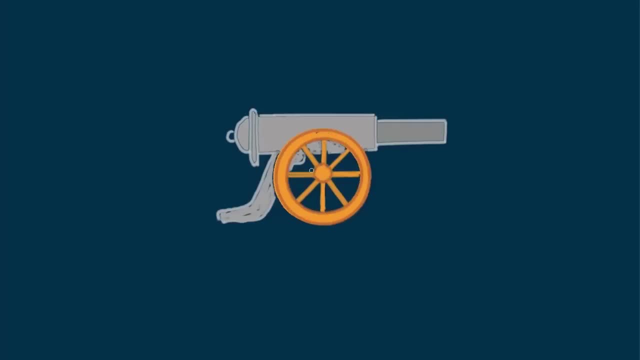 Now consider a cannon being fired. Let's look at a snapshot of the ball part way down the barrel. While a force pushes the cannonball, an equal and opposite force pushes back on the cannon, which causes its recoil. Since this pair of equal and opposite forces occur for the same length of time, the impulses 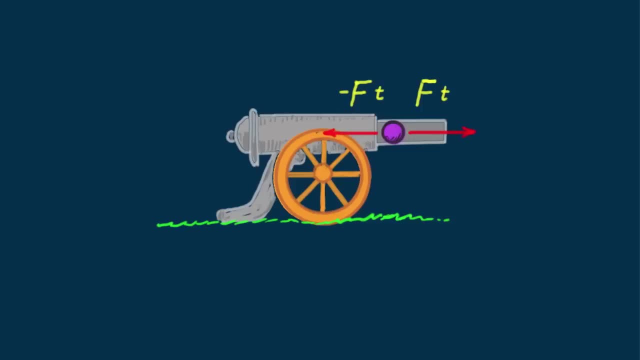 are also equal and opposite, So impulses relate to Newton's third law. This pair of impulses is internal to the system consisting of the cannon and the cannonball. Internal impulses don't change momentum. They change the momentum of the system Before firing, the system's at rest and the momentum is zero. 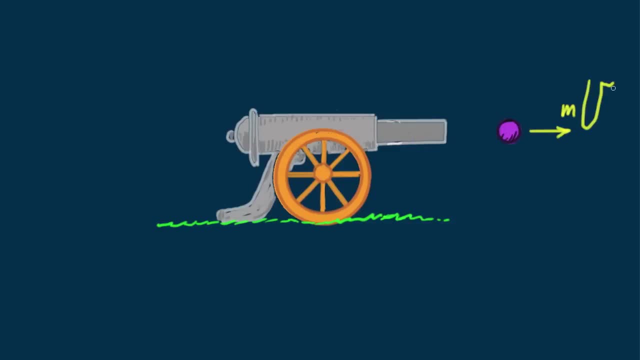 After the firing, the net momentum or total momentum is still zero. You can imagine the cannon recoiling somewhat to the left with the same amount of momentum as the cannonball. Net momentum is neither gained nor lost. So we see, the cannonball's momentum is mainly velocity, while the cannon's momentum is. 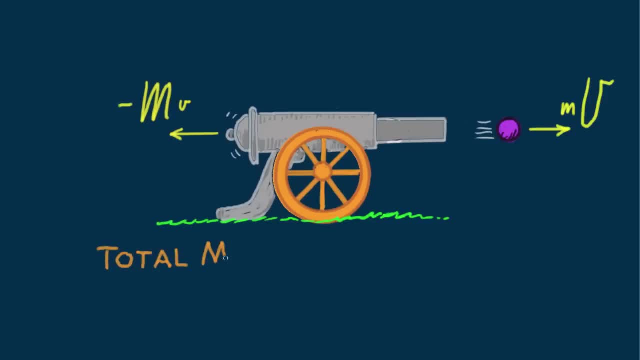 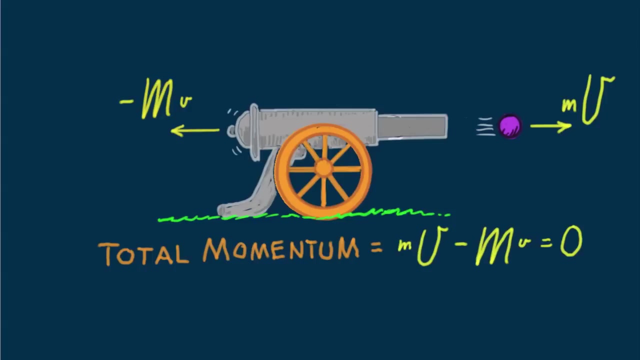 mainly mass. So although both the cannonball and cannon each have momentum in the combined cannon-cannonball system and being vector quantities they cancel to zero. We say total momentum is unchanged, zero before firing and zero after firing. In any interaction where no external impulse is exerted, momentum remains unchanged. 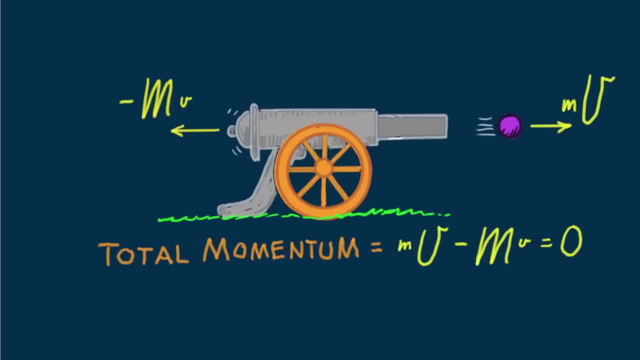 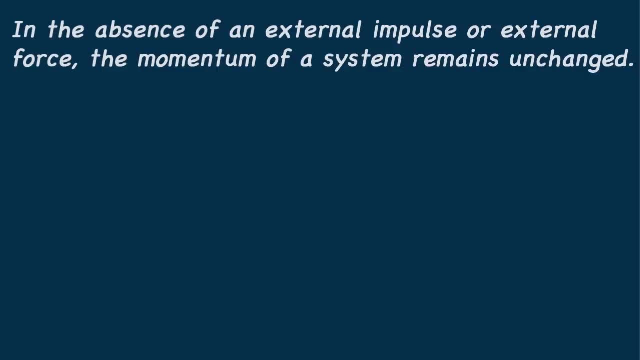 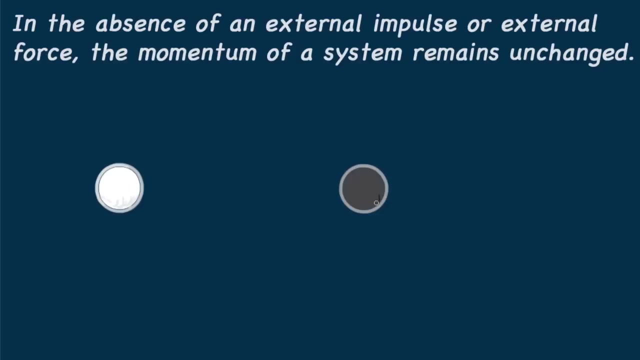 We say momentum is conserved. We call this the conservation of momentum. In the absence of an external impulse or external force, the momentum of a system remains unchanged. Momentum conservation and the role of systems are nicely illustrated in the game of pool. I think we've all marveled how a cueball comes to a halt when it collides head-on with its 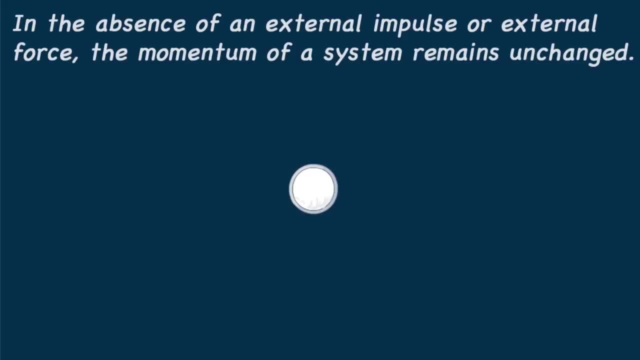 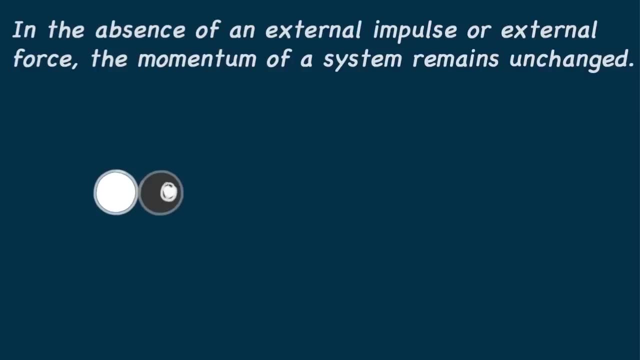 cannon head-on with a stationary 8-ball transferring its motion to the 8-ball When contact is made. consider the system consisting only of the 8-ball, the 8-ball system. When a cue ball strikes, there's an external force on the 8-ball which then gains momentum. 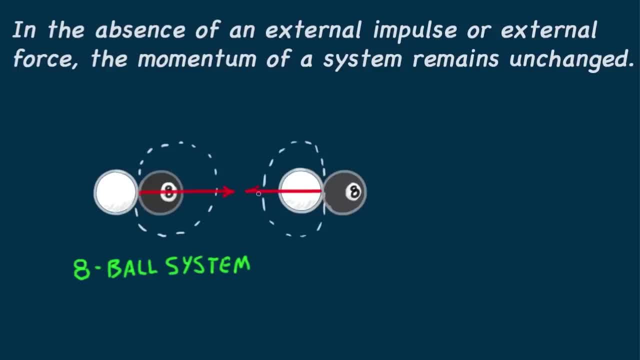 Let's look at this from the point of view of the cue ball system. When the cue ball strikes the 8-ball, a reaction force by the 8-ball which is external to the cue ball system changes the momentum of the cue ball. 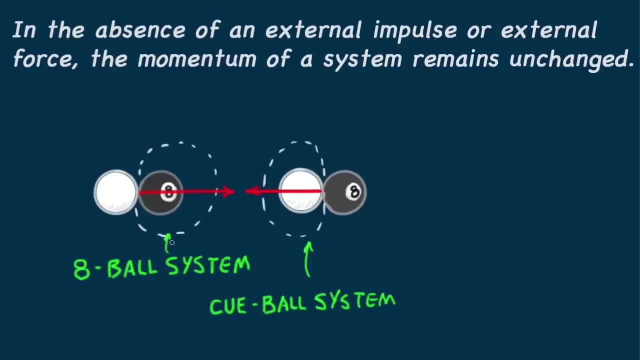 It brings the cue ball to a halt. Now let's look at this from the point of view of the combined 8-ball cue ball system. In this larger system, the forces we've considered are internal forces. No external force acts on the system. 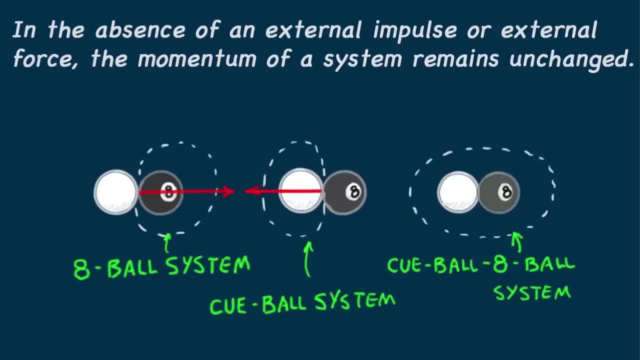 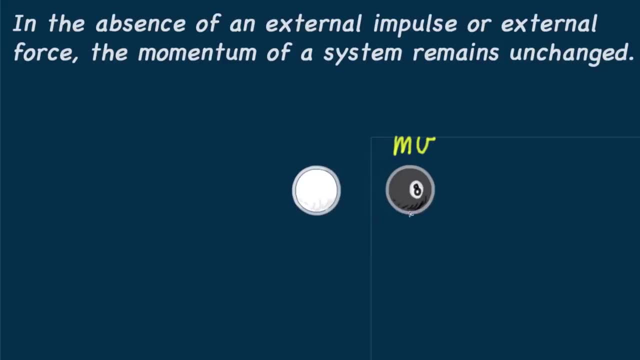 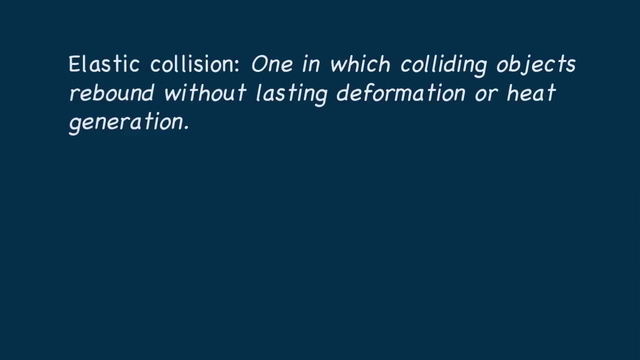 So there is no net change in the system's momentum. The momentum before the collision was mv and the momentum after the collision is still mv. Momentum has simply transferred from the cue ball to the 8-ball. The cue and 8-ball illustrate an elastic collision. 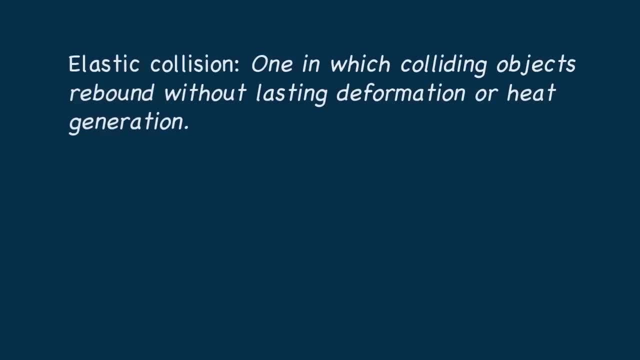 That's one in which colliding objects rebound without lasting deformation over time. The cue and 8-ball illustrate an elastic collision. That's one in which colliding objects rebound without lasting deformation over time. The cue and 8-ball illustrate an elastic collision. 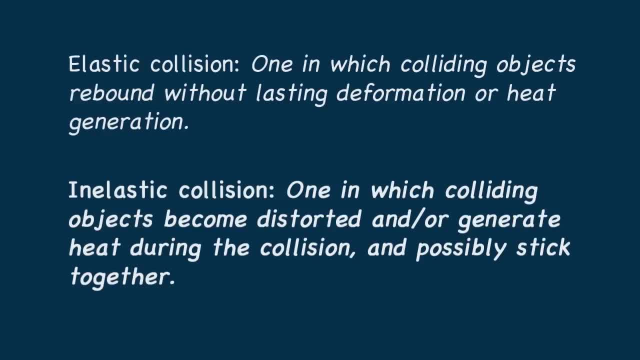 The cue and 8-ball illustrate an elastic collision, That's one in which colliding objects rebound without lasting deformation over time. And then there's inelastic collisions, where colliding objects become distorted and or generate heat during the collision and possibly stick together. 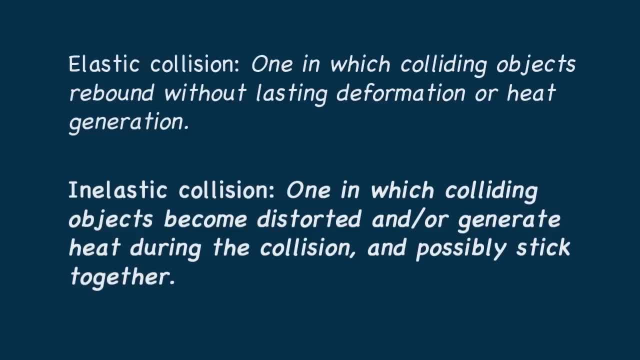 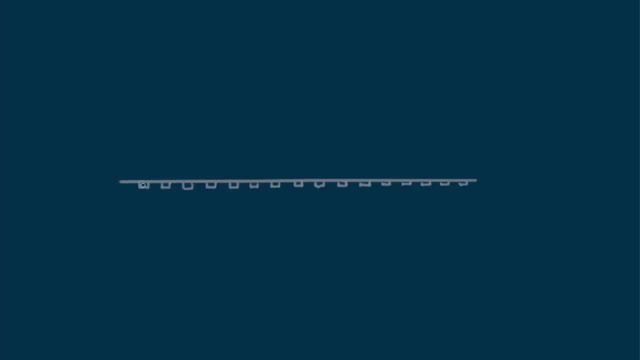 Here's the important thing: Momentum is conserved in all collisions, whether they are elastic or inelastic, so long as no external forces act during the brief period of collision. I want to leave you with a question: Is theубanks being elastic or inelastic? 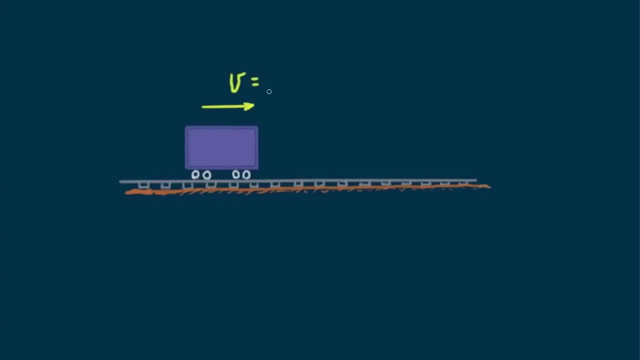 Suppose a freight train car rolls along a track at 10 meters per second and collides with an identical freight car of the same mass. at rest The two cars couple together and move as one along the track. How fast do the couple cars move? Think about that. Until next time, good energy.